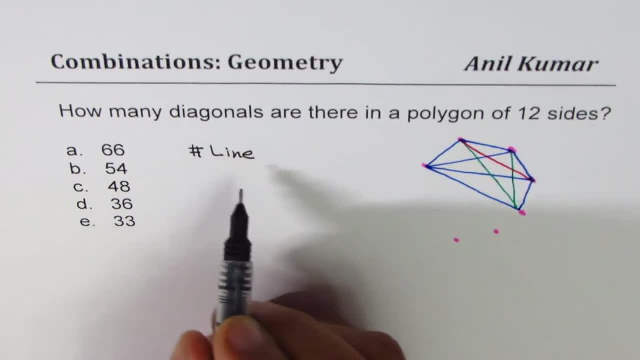 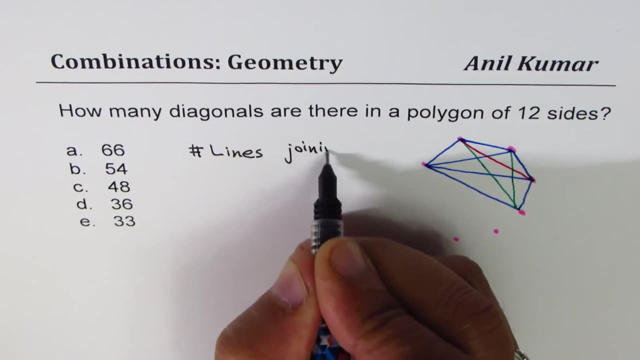 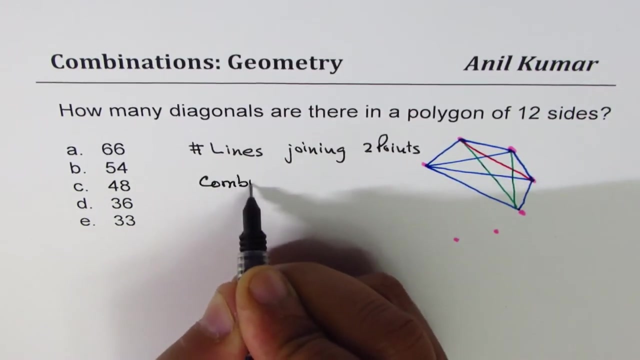 So we say number of lines could be formed with two points. So number of lines is joining points, right. Joining two points, Is that okay? So that is combination, right. So that is combination Using two from n- right. So that is what the result is And that gives you total combination. 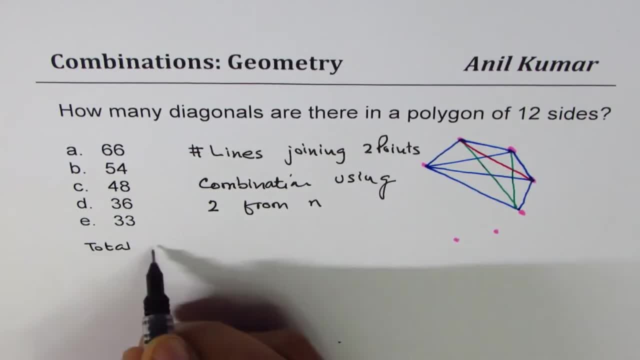 of lines, right, So we can write here total number of lines. Since we have 12 points, we'll straight get to the question. now You've understood the concept right: 12c2.. So 12c2 is the total number of lines that you can draw. So out of these, what we see is out: 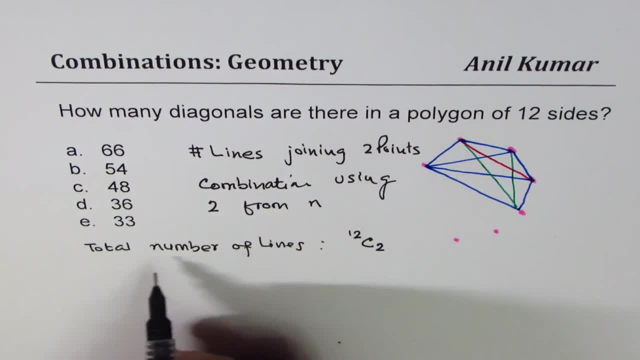 of n will be the sides of the polygons, right. So how many are diagonals right? How many are diagonals? Can you tell me that? How many are diagonals? So we have to take the edges Right. So from 12c2 we take away 12.. Because we don't actually take the edges, So we take theこれ. edge right away. This is negative. So the upper edge here is negative, This one we take away It is right, And then from the bottom we take 12c2.. And from the bottom it is above, And then took 12c2.. And then from the top we take away 12ставляedve, and then up to the end we take the. 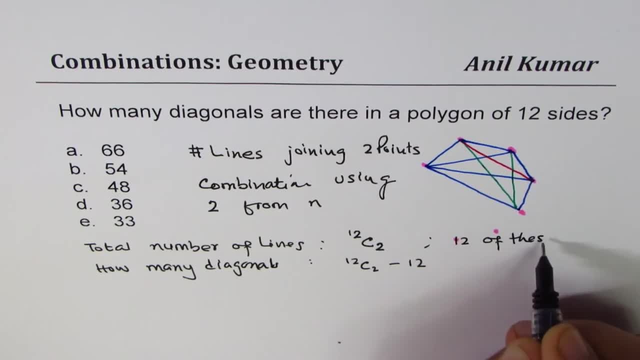 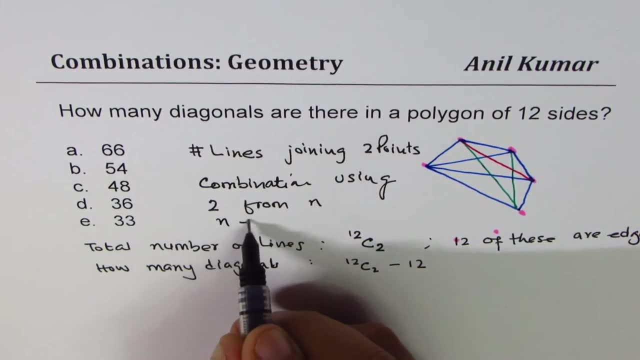 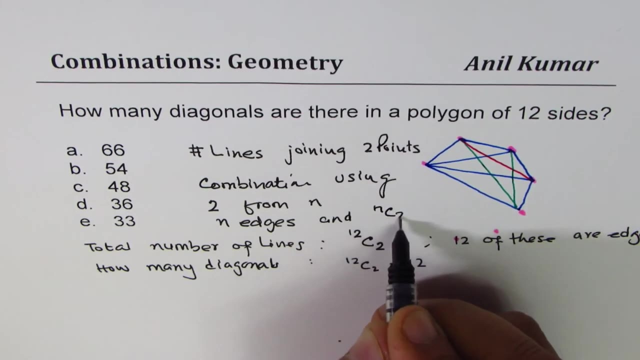 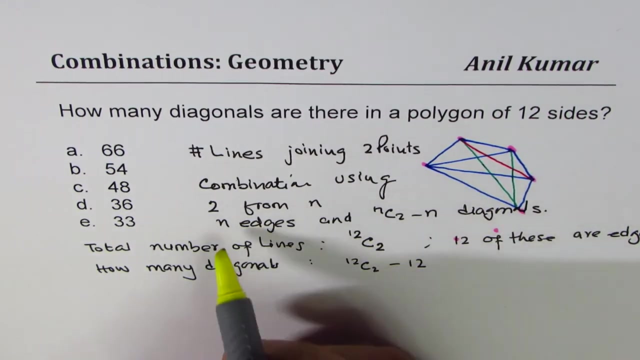 12 of these are edges right. So for n we have n edges and nC2 minus n diagonals. Does it make sense? So that is how we could get our formula, Do you understand? So there are n edges for a polygon with n vertices. 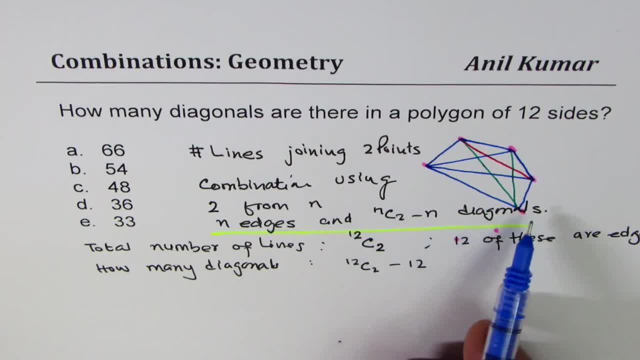 nC2 is total number of lines, So their difference is the number of diagonals. Rest is that okay? So that is how we can find the answer. So 12C2 minus 12.. So 12C2 will be 12 times 11, times divided by 2 minus 12, correct?